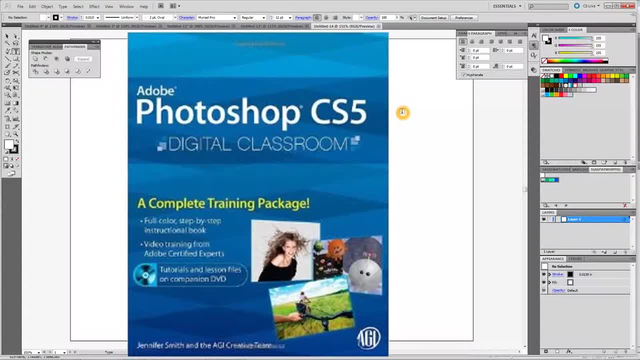 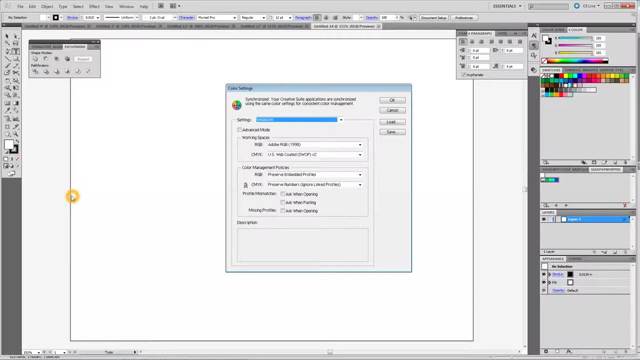 I'm going to talk about color gamuts in a minute. A lot of this information you can read about in that book. You can buy that book on Amazon for like nothing. now It's. I'll put a link below. Okay, let me just tell you what I'm doing. I'm going to edit color settings. This whole video did not come from her book. I've worked on it for a while So, but if you're trying to learn this and you want a lesson, her book is a good book to use. Okay, this panel right here says: 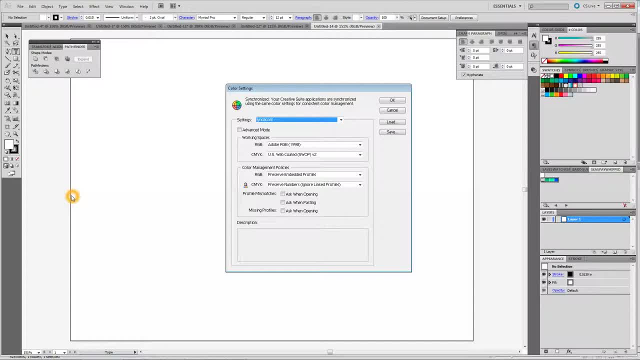 I've worked on it for a while, So but if you're trying to learn this and you want a lesson, her book is a good book to use. Okay, this panel right here says: I've worked on it for a while, So, but if you're trying to learn this and you want a lesson, her book is a good book to use. Okay, this panel right here says: 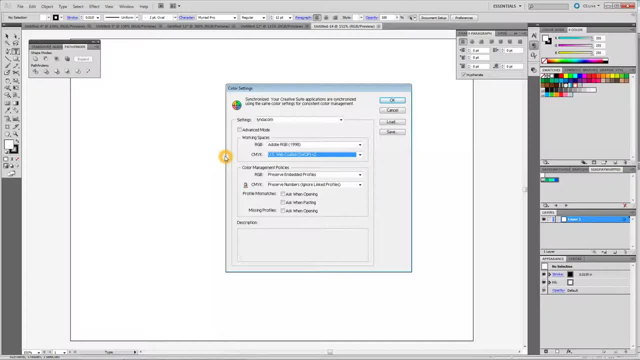 I've worked on it for a while, So but if you're trying to learn this and you want a lesson, her book is a good book to use. Okay, this panel right here says: I've worked on it for a while, So, but if you're trying to learn this and you want a lesson, her book is a good book to use. Okay, this panel right here says: 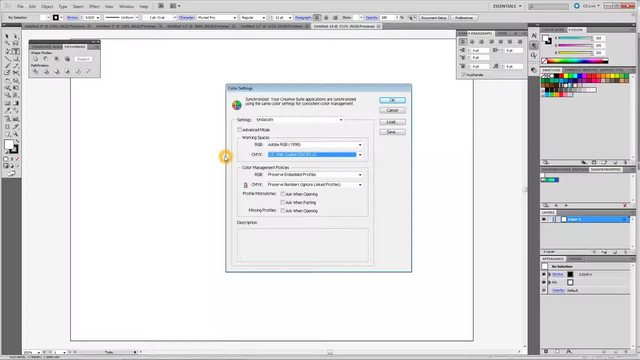 I've worked on it for a while, So but if you're trying to learn this and you want a lesson, her book is a good book to use. Okay, this panel right here says: I've worked on it for a while, So, but if you're trying to learn this and you want a lesson, her book is a good book to use. Okay, this panel right here says: 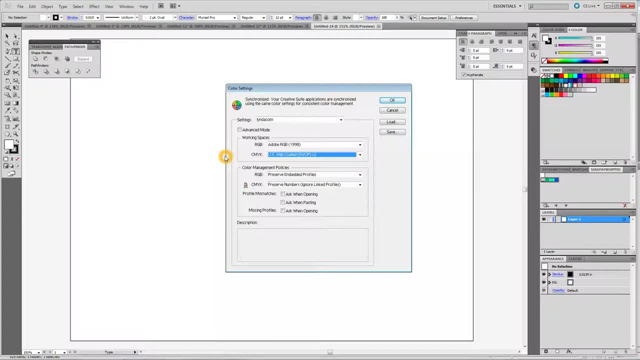 I've worked on it for a while, So but if you're trying to learn this and you want a lesson, her book is a good book to use. Okay, this panel right here says: I've worked on it for a while, So, but if you're trying to learn this and you want a lesson, her book is a good book to use. Okay, this panel right here says: 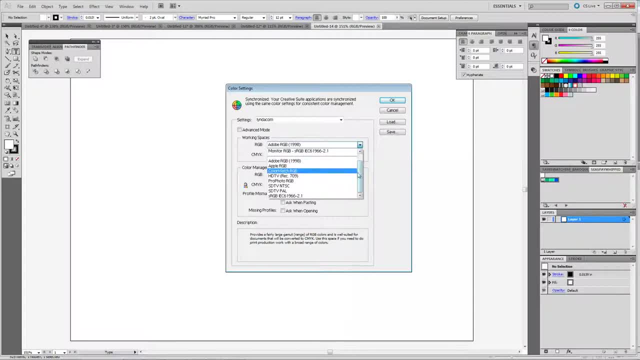 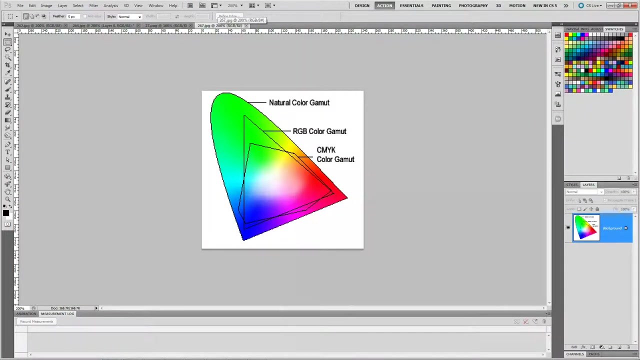 I've worked on it for a while, So but if you're trying to learn this and you want a lesson, her book is a good book to use. Okay, this panel right here says: I've worked on it for a while, So, but if you're trying to learn this and you want a lesson, her book is a good book to use. Okay, this panel right here says: 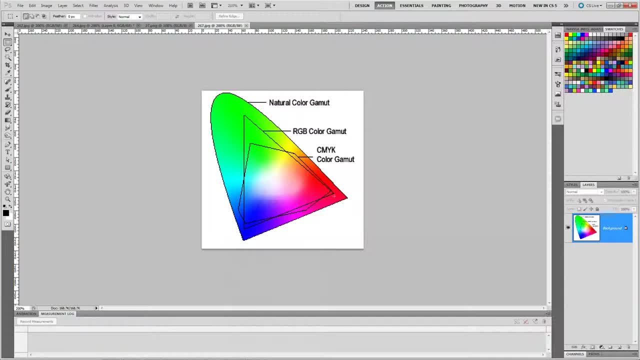 I've worked on it for a while, So but if you're trying to learn this and you want a lesson, her book is a good book to use. Okay, this panel right here says: I've worked on it for a while, So, but if you're trying to learn this and you want a lesson, her book is a good book to use. Okay, this panel right here says: 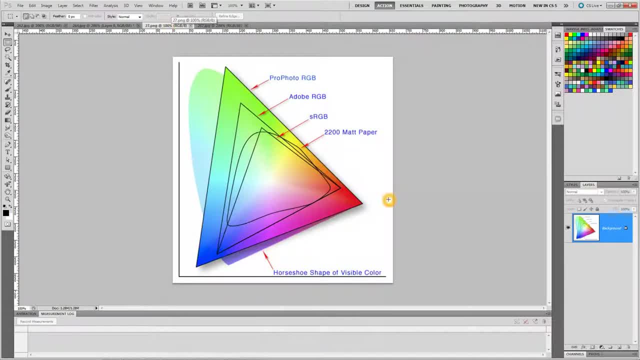 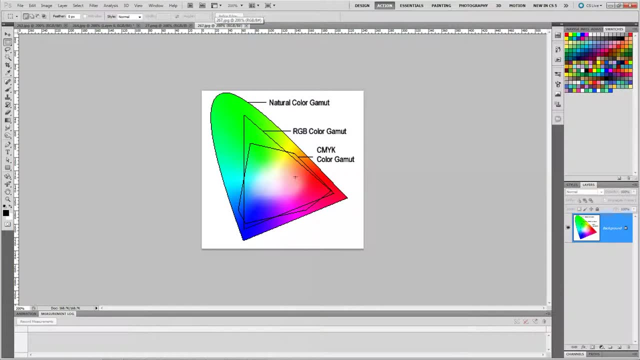 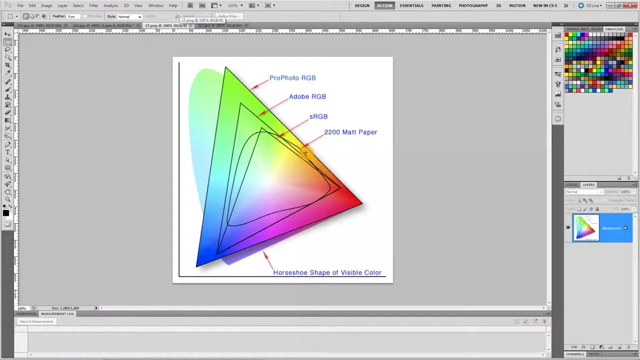 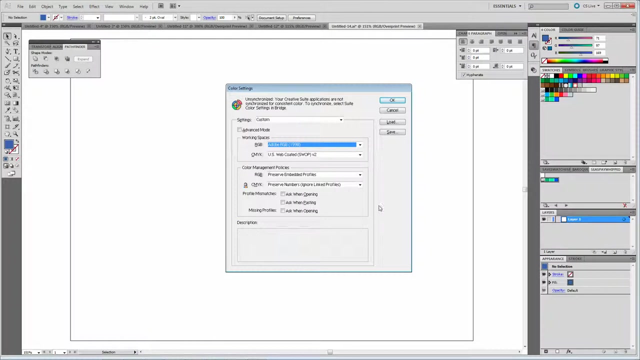 I've worked on it for a while, So but if you're trying to learn this and you want a lesson, her book is a good book to use. Okay, this panel right here says: I've worked on it for a while, So, but if you're trying to learn this and you want a lesson, her book is a good book to use. Okay, this panel right here says: 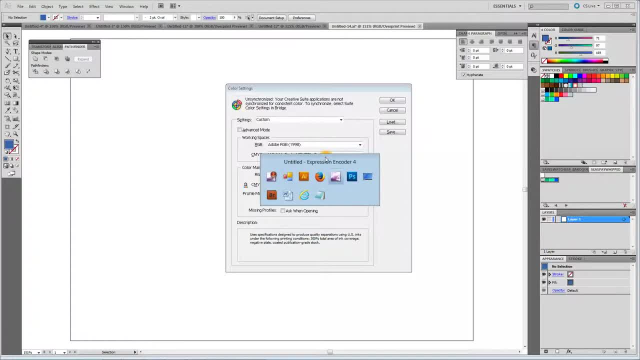 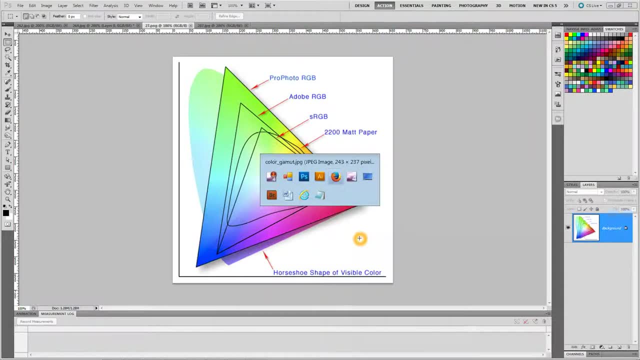 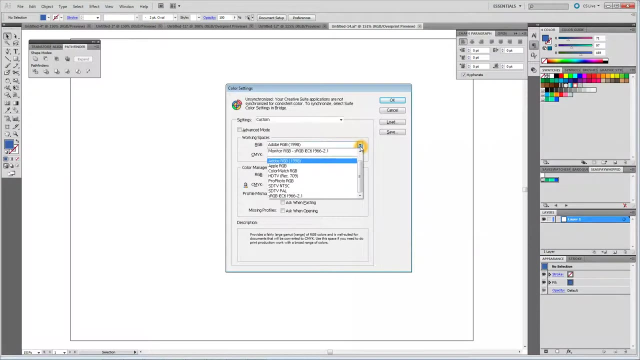 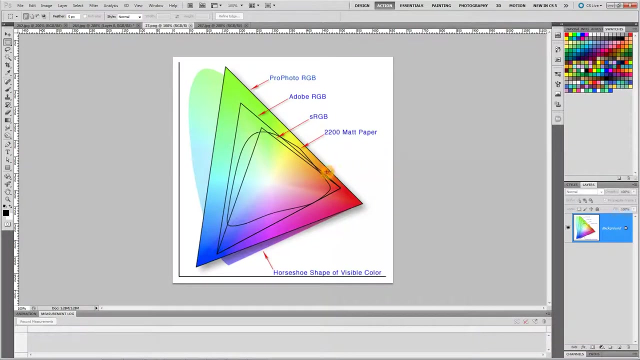 I've worked on it for a while, So but if you're trying to learn this and you want a lesson, her book is a good book to use. Okay, this panel right here says this: rgb color gamut, color space srgb- right here. okay, so that's how that works and what that 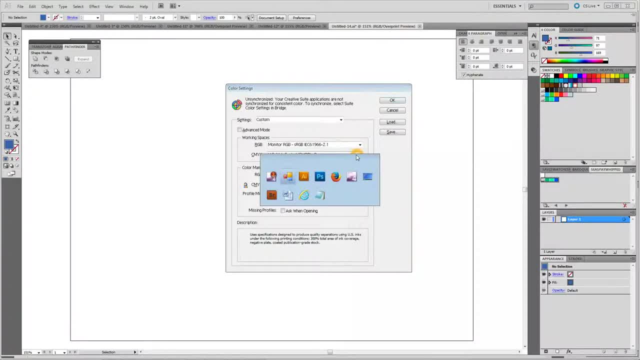 relates to when you are choosing these. this is what you are, this is what you are choosing this. okay, i hope that explains it to y'all. it took me a long time to grasp that and it seems so simple now, but i really did struggle with it. so it's not just the rgb, you've got color gamuts. 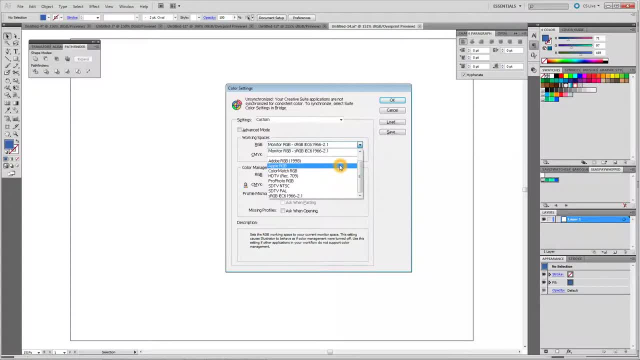 with inside the rgb, and each of these color gamuts represent different shades of color and different things, so you need to consider those. hope that helps. and when i was starting out, i'm just being honest, i didn't understand what gamut is and for you, those of you that are in that boat, 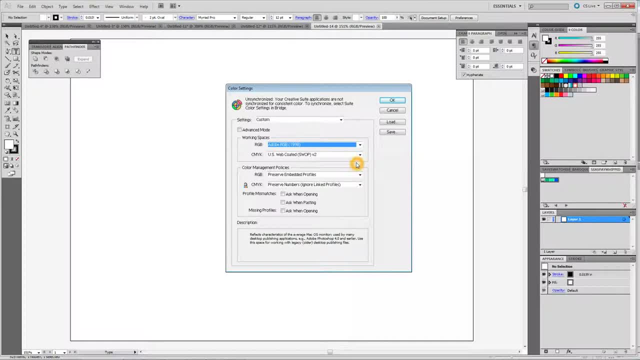 a gamut represents the numbers of colors that can be detected or produced on a specific device. um, so this is the. this has a different number of colors that can be produced than this does. okay, so a gamut is a range of color. even though you pick rgb, you can't get all the rgb ranges. 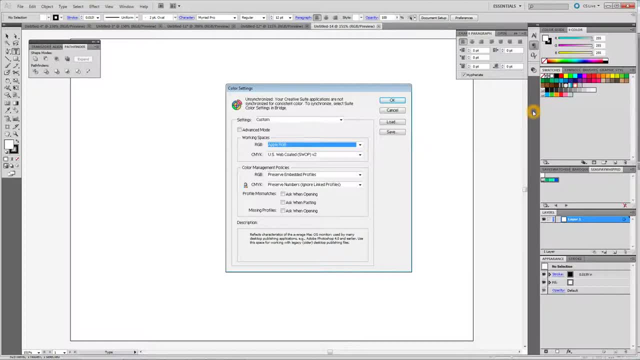 okay, um, so that's that. now there's another thing about this um menu item i want to talk, talk to you about here. it says unsynchronized. your creative suite applications are not synchronized for consistent colors. to synchronize select color settings and bridge: okay, this you really, really want to do. when you get going on um your creative suite, you're going to be using 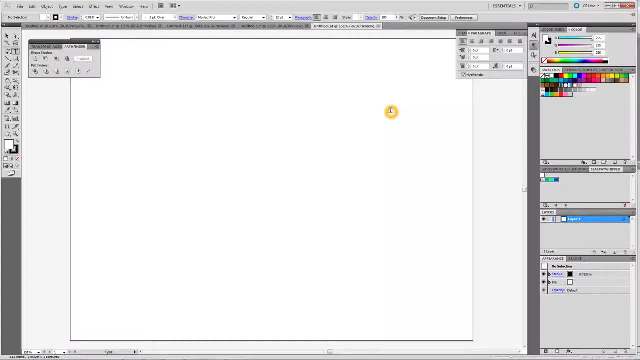 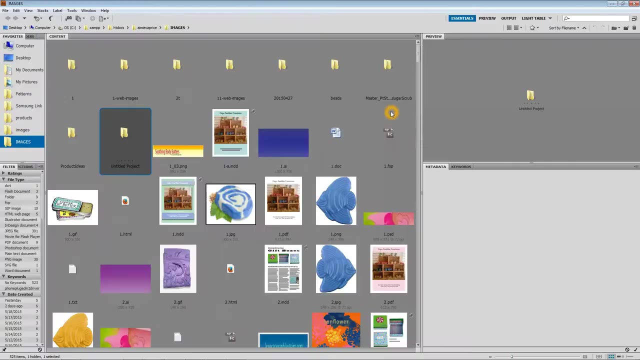 photoshop and cutting things and slicing things and bringing them into illustrator and vice versa, and you want the color you produce in one application to match the color you produce in the other application. so in order to do that, you want to go to bridge and do your color settings there so that they are consistent um across all your applications. 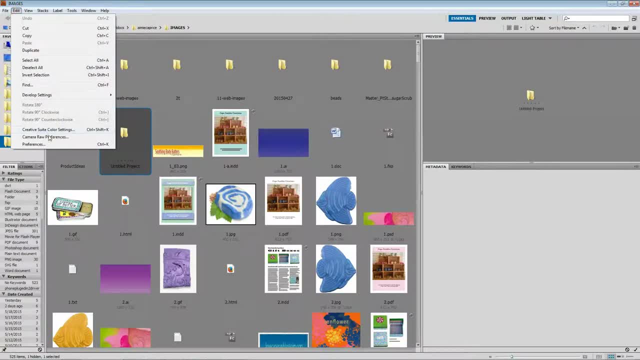 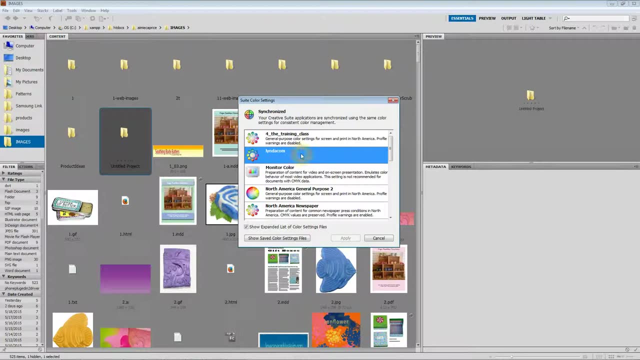 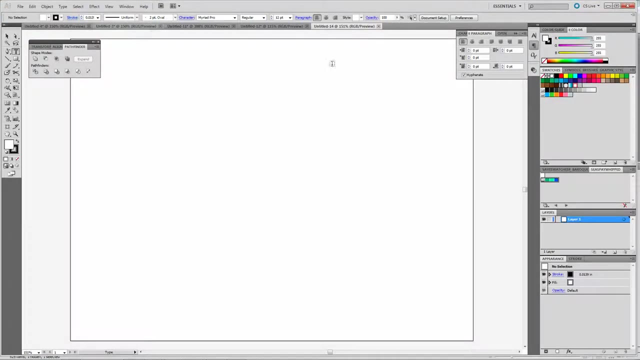 and if you go here and you go to edit and then you hit creative suite, color settings- and this one i created on my own is a personal one, and so that's what i usually use- and then if you go now, this i've changed for the sake of us talking. 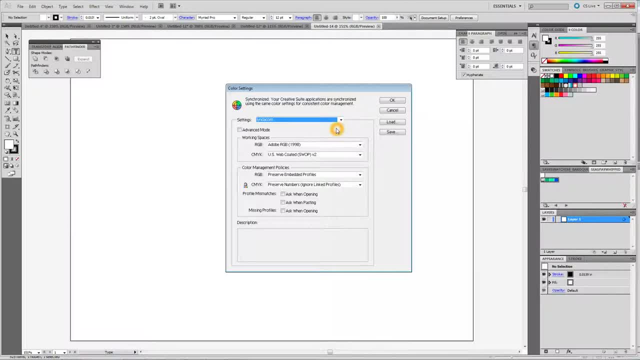 so it's synchronized now. okay, so if i open up photoshop, it too will be synchronized and they will all have these settings. and the settings is a synchronized um color setting for your creative suite applications- flash, photoshop, indesign, illustrator, whatever you're using, but they will all have consistent color. uh, setting. 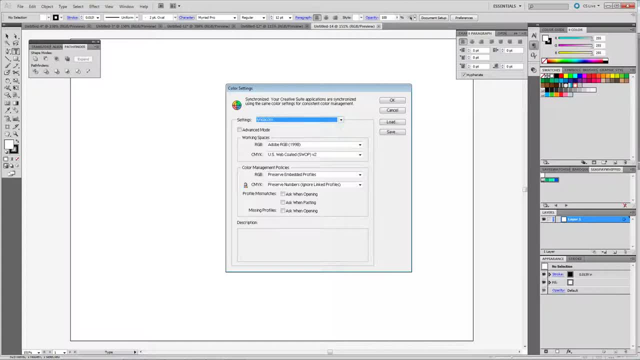 profiles. so if you open up um photoshop, you will see that it has this, um it has this working space or adobe rgb and this uh working space, uh, the cmyk working space, and you will see that across all applications. if you open up my flash, they will have the same thing. they all open up with uh this. 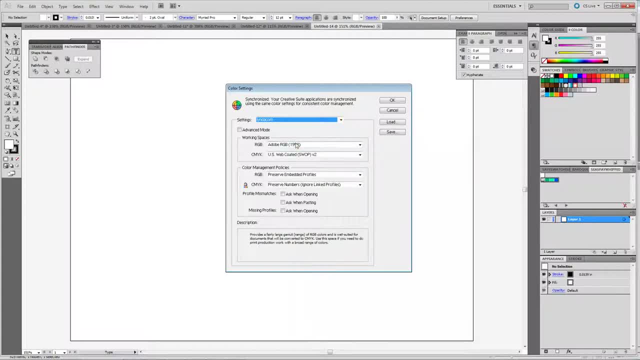 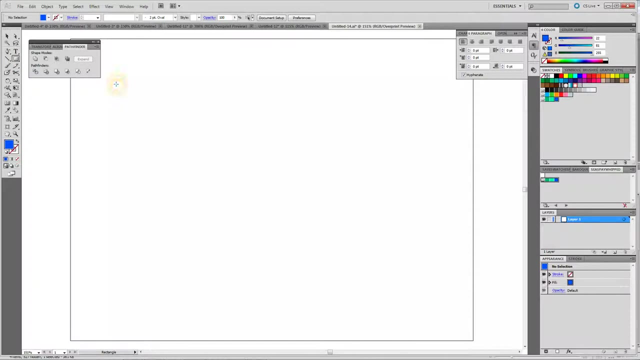 color setting. this color setting pre-defines these options here for you, so you don't have to do that. um, there's also a couple standard ones, but, um, that's the one i use. now let's look at the color picker. going to the tools menu, i'm clicking on the rectangular marquee right here and i'm drawing. 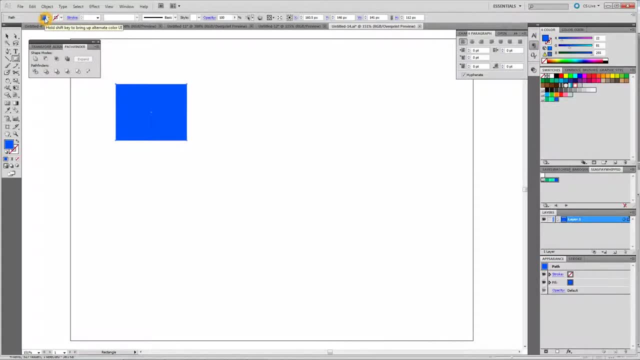 out a square of color. it's blue. because this is blue and it has no border because this has no border. if you double click this icon in the tool menu on the left hand side, you get what is called the color picker. the color picker is very informative in helping you do your color management. 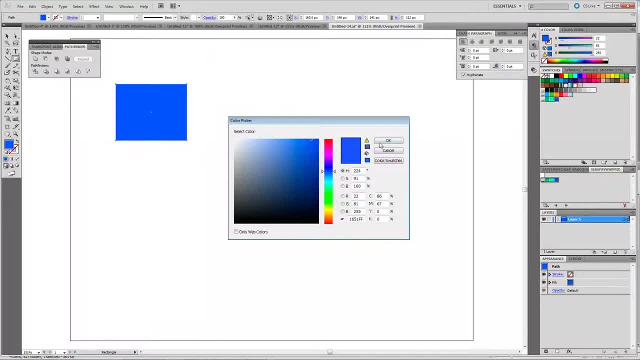 this right here is: this is your out of gamut for printing warning icon. this indicates that, although you may have selected a very nice color, it's never going to print based upon the preset color setting you selected. to fix that, illustrate illustrator makes that very easy. all you have to do is click on. 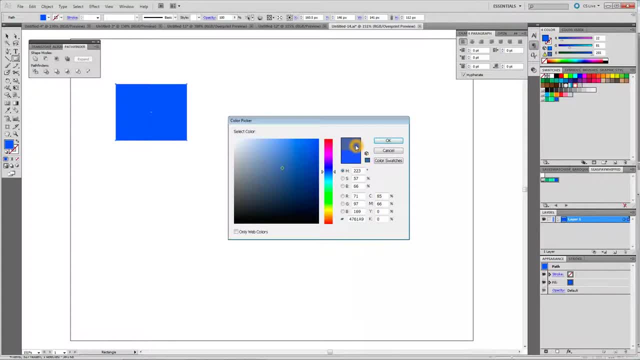 it and it says, okay, down here is the original color, up here is the new color it's selecting, so that this color will be in gamut of um, your color printer. you hit ok if that's all you want to fix, and it will lay that color down. see how it did that. now let's go. 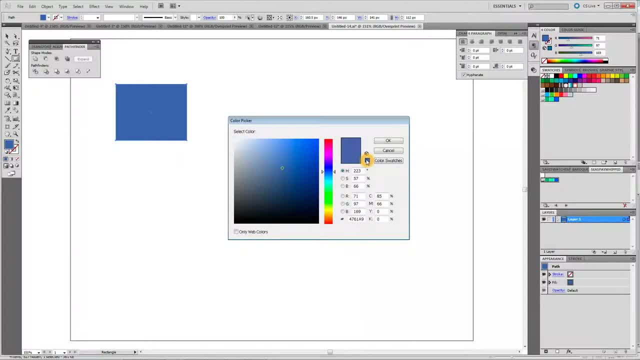 back into it. you still have some other issues going on. right here is um another warning, and what this is saying is that it's not a web safe color. this color that i've chosen, now that it's in gamut with my printer, is still not um. 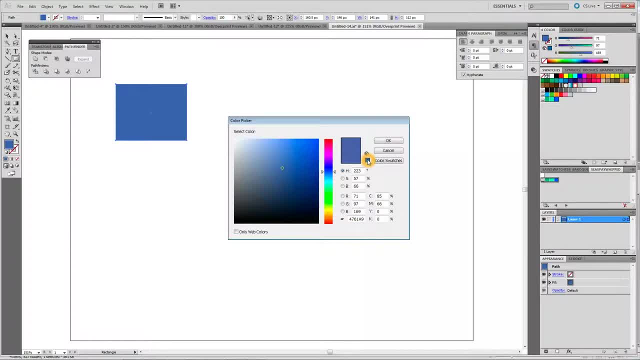 going to be a color web safe, uh, web safe color. to fix that, all you have to do is click on it. illustrates illustrator, photoshop, whatever you're using, fixes it for you, makes it very easy. this is the color you were at. this is the new color. if you're happy with it, hit ok. now there's. 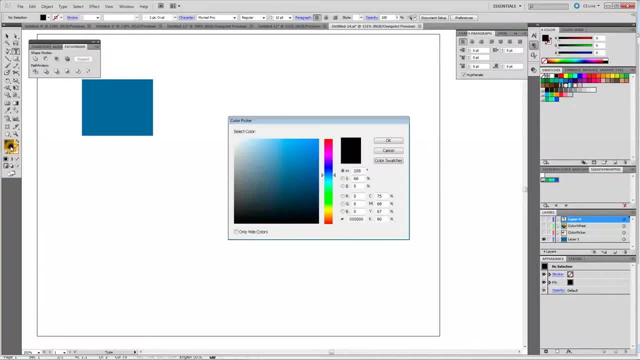 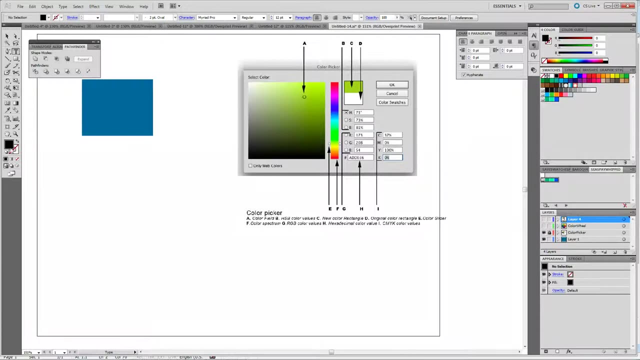 some other elements, um, that we want to look at in the color picker. let's start with. i've made this on diagram over here. let's open that up. I don't know, hang on one minute, let me see if I can get this opened. okay, good, so I want to move this over here. there's some. 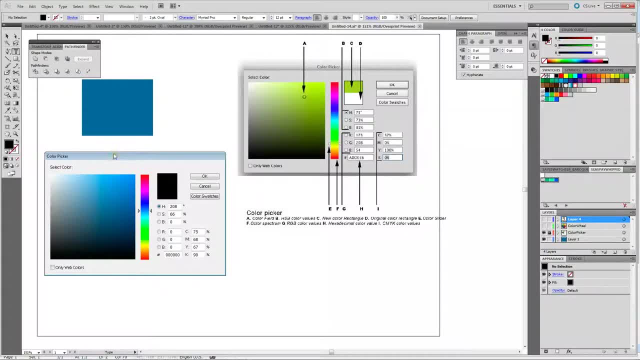 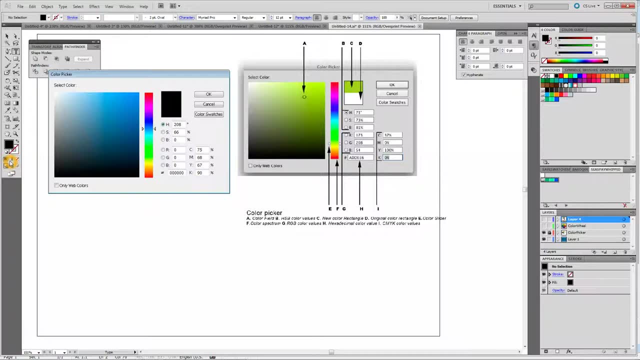 other elements. this is just an image you all. this is the actual color picker, and this is just an image I made. there's some other elements in the color picker window that we want to talk about, and one is this area right here. this is called the color field, and as you click on it, your, your color comes up, and it'll. 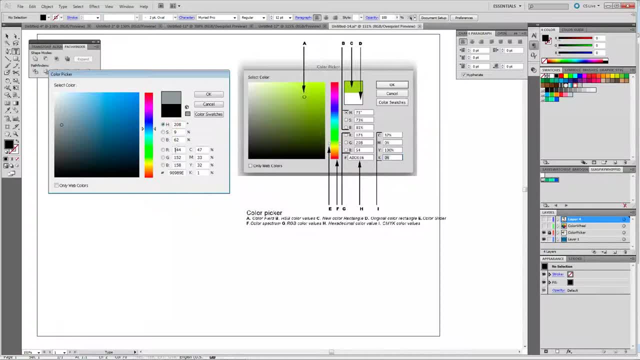 show you what the colors are. also know that. notice that these things change. the values in these boxes change. if you want to use colors that are safe only for the, that are safe for the web devices, you can check this box and it will give you only colors that are color web color. what are they called? color safe? color web safe. 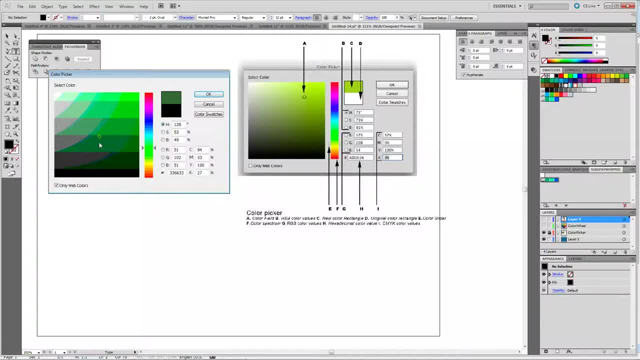 colors. so if you want this hue, these are: these are green in the green hue. these are colored safe colors in the orange hue. these are color safe colors. our web safe colors is what I'm trying to say, and vice versa. so that's how that that works. so if you're doing web design, you really want to have this on, if you're. 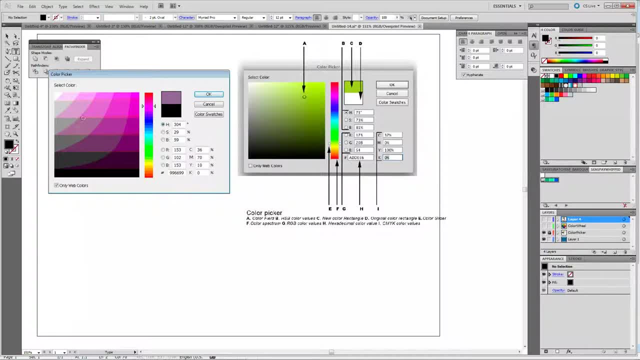 designing for a web application, because all these colors are, say, web safe colors and they will produce consistently across applications, which you really want. ok, now let's talk about some of the other components in this window over here, you have a button called color swatches. if you click on it and it will. 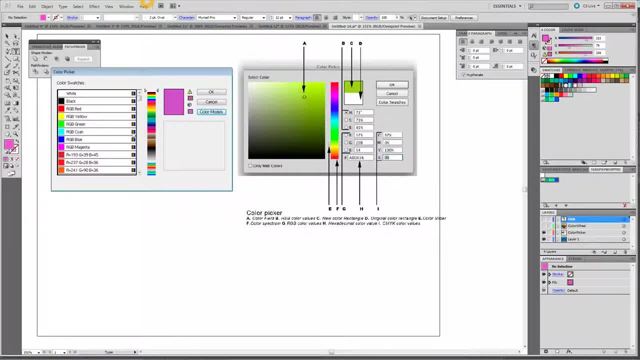 give you all your swatches that are in this panel as well. this little icon indicates that you are in red, green, blue module. you can pick colors from there again. you have your web safe and a gamut safe warnings right here. i'm over here. you've got the numbers that this color represents and CMYK mode. 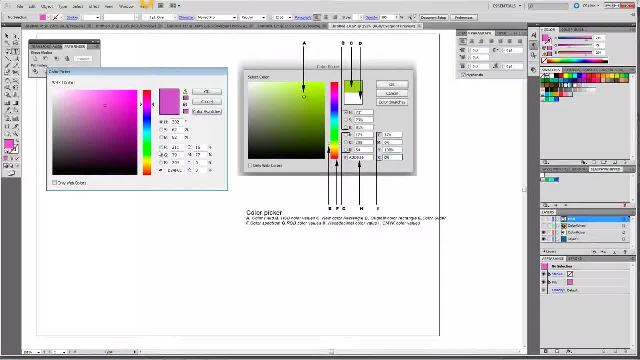 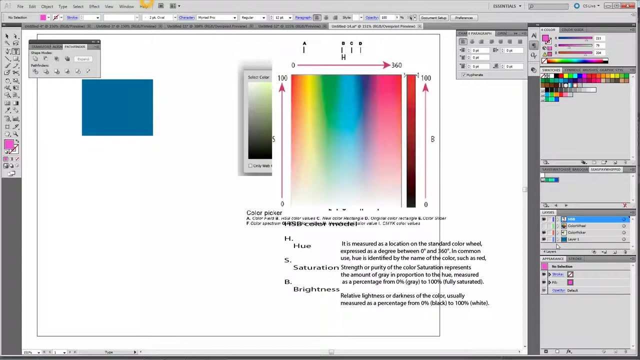 or model. here you've got the red, green, blue that this, the numbers that this color, that work you're currently on, represents in the RGB model. up here you have the HSB model. if y'all hang on for just a moment, I have another little picture for y'all to look at while I explain some 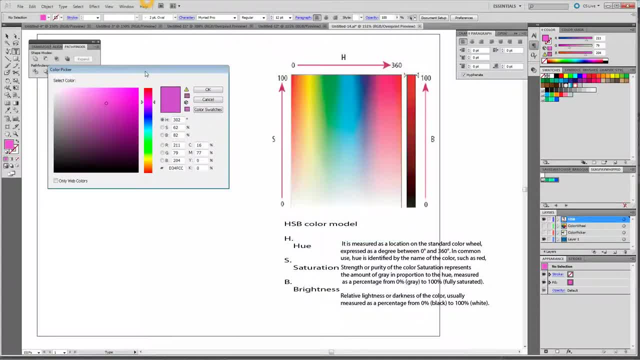 things to you here. these are just diagrams I made real quick in Photoshop so that we could go over this stuff. HSB stands for hue, saturation and brightness. if you look down here on the right hand corner of my screen, you'll see that this is the HSB model. this, this color that's selected is. these are the: 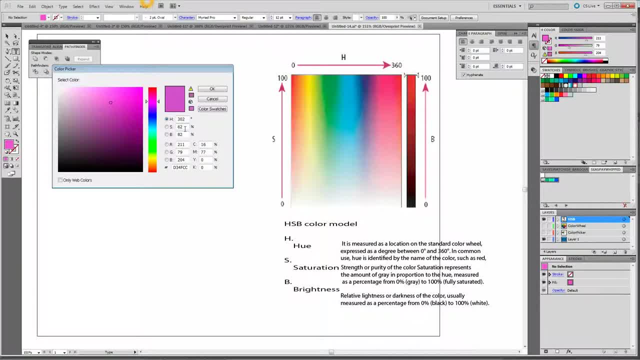 numbers that pertain to that in the HSB model: hue is this? okay, these are hues: pink, red, green, orange, those are hues here is represented in a degree and that's because on the color wheel, if you look at a color wheel is a circle and it's. 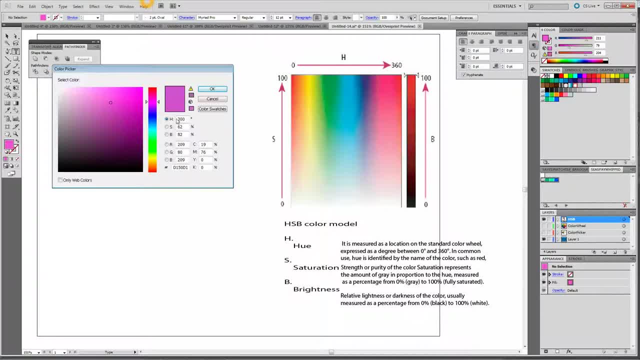 360 degrees. so that's telling you where on that color wheel that color is all the way up to 360. see what I'm saying there, and if you read down there, it says that as well. I've got another picture for that. hang on for one minute. let me close this, okay. 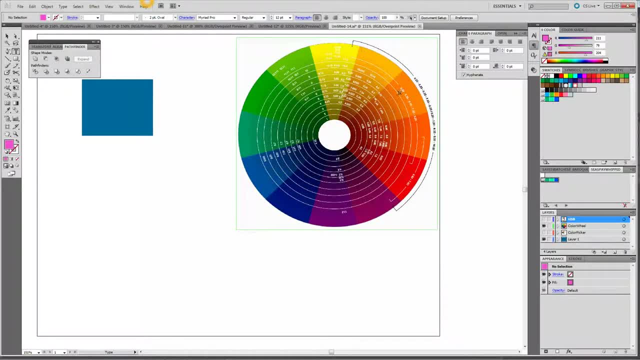 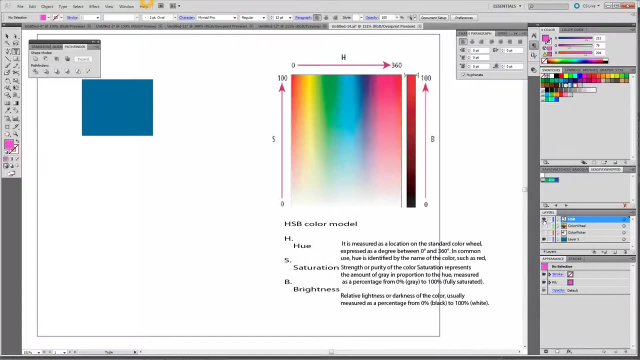 here's a color wheel. as you can see, it's 360 degrees. that number is in degree format because it's telling you we're on the color wheel degree wise. it, it lays or it falls. I guess it's the correct term to say there. okay, let me get my thing back over here. 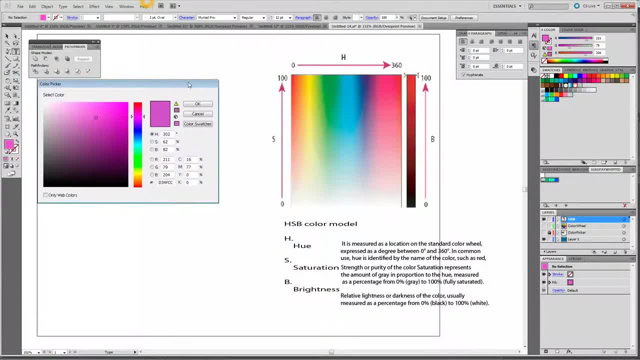 up in here. okay, so that takes care of hue. next component on here is saturation, and saturation is very simple: the purity, and it's represented by percentages. this is a hundred percent. that's the most saturated you can be of that color. this is zero percent. that's the least saturation you can be in the color. so it 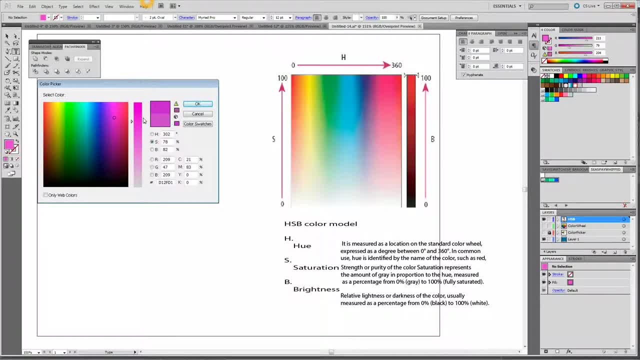 is the strength or purity of the color. saturation represents the amount of gray in proportion to the hue and, like I said, it's measured in percent. zero percent is gray, hundred percent is your full saturation. okay, next component on here is B, and if you look down here, in the right hand corner, B stands for: 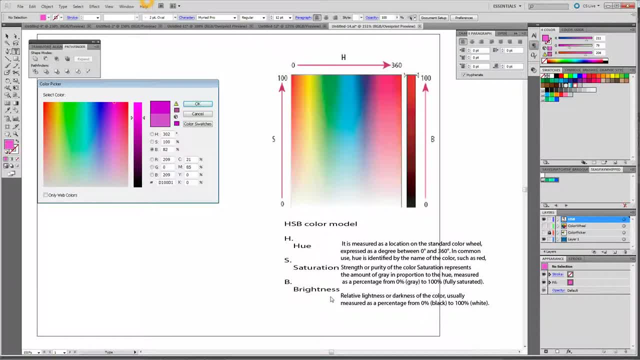 brightness. but I will tell you, I think of B as black. it's in my mind how much black is being laid down. so here again, it's in percentages. the number is represented in percentages. the technical book term says that B stands for brightness and it's lightness or darkness of a color. so 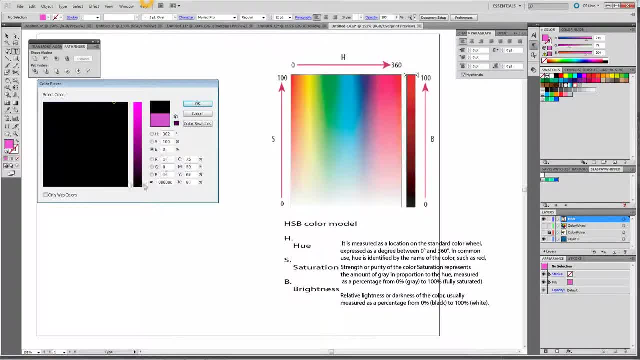 that's a hundred percent light, and that would be zero percent, which is black light, no light. okay, so that's how. that's how the HSB model works. that's all I've got for you all for now. the photoshop, adobe photoshop, cs5 digital classroom by Jennifer Smith is a good book if you.